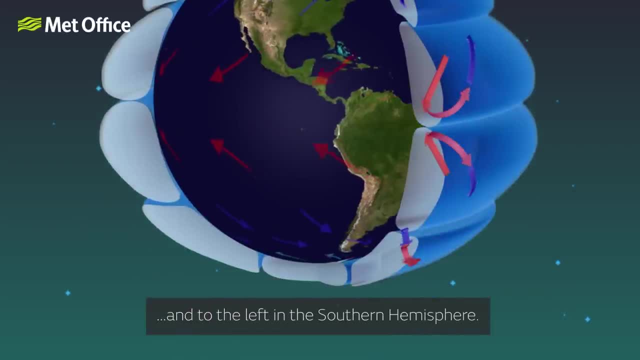 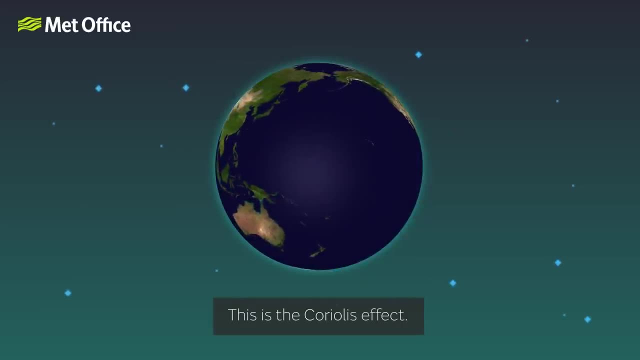 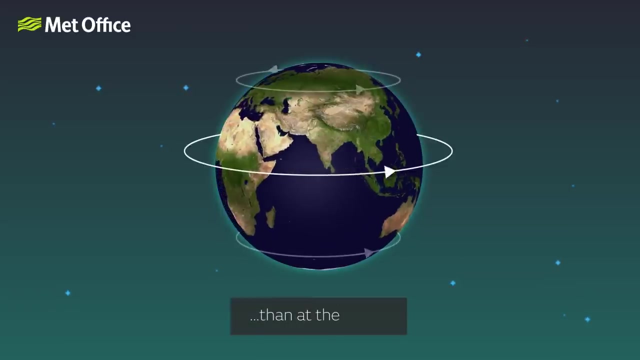 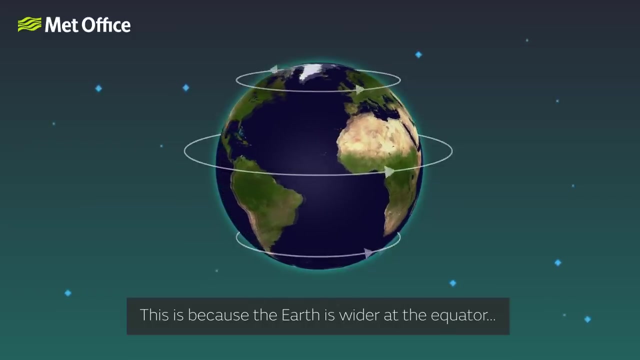 hemisphere and to the left in the southern hemisphere. This is the Coriolis effect. The key to the Coriolis effect lies in the fact that the earth's surface rotates faster at the equator than at the poles. This is because the earth is wider at the equator, so has further to travel in one day. The result of 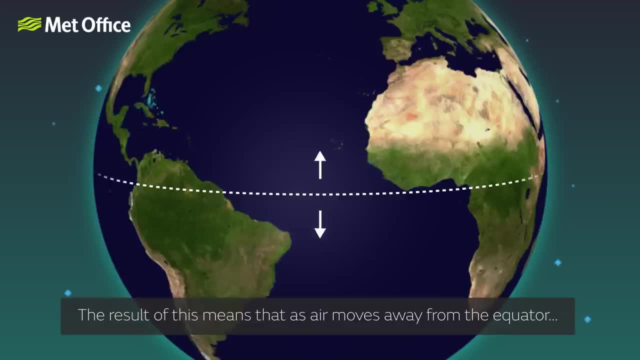 this means that as air moves away from the equator, it doesn't move in a straight line relative to the earth's surface. Instead, it appears to an observer on the ground to move in a slightly curved direction, but there is no physical force causing this deflection as the atmosphere. 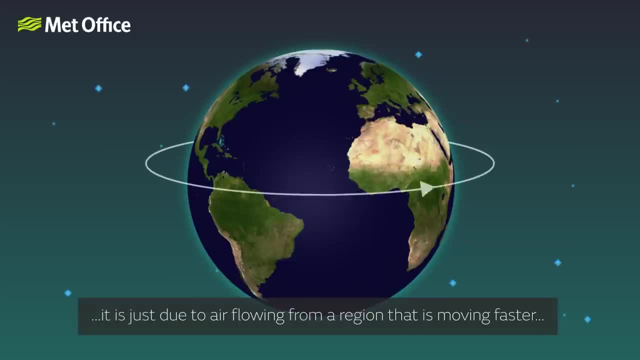 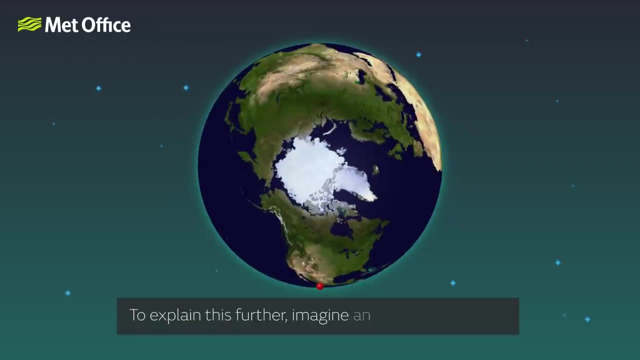 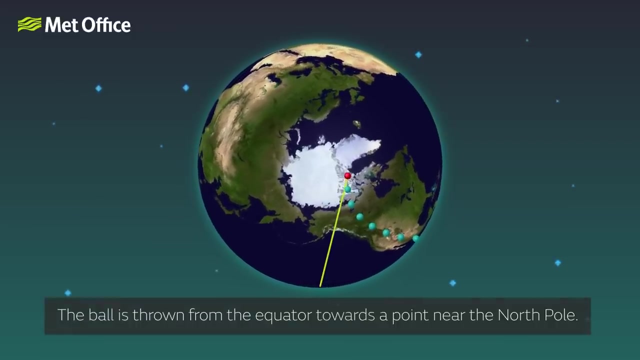 rotates with the earth, It is just due to the air flowing from a region that is moving faster to a region that is moving more slowly. To explain this further, imagine an air parcel as a ball. The ball is thrown from the equator towards a point near the North Pole. 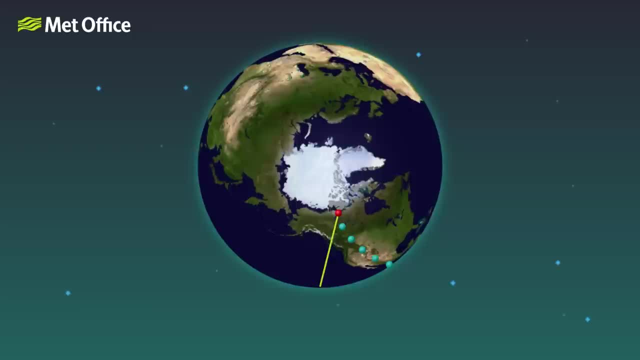 Even though it moves in a straight line, the ball will appear to an observer on the ground to curve away and land to the right of its target. As the points near the point of focus hit the ground, the ball will rotate and in a straight line it moves from one side of the sea to the other. 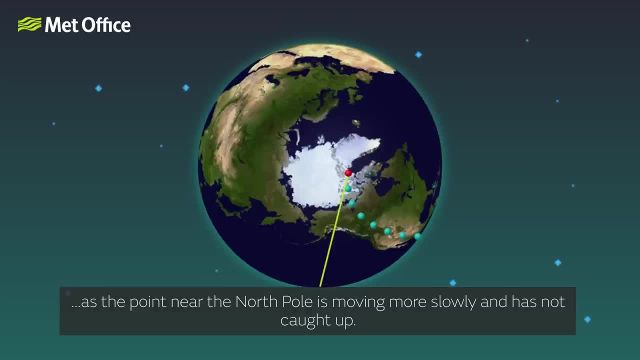 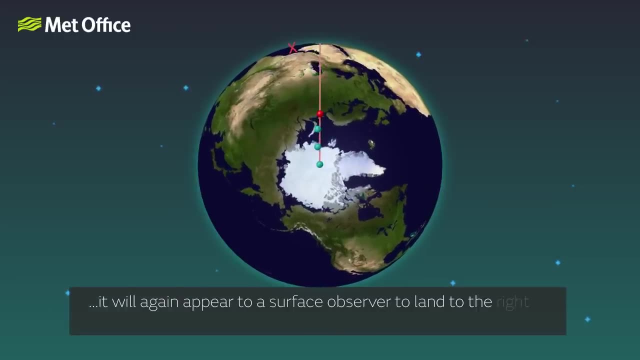 North Pole is moving more slowly and is not caught up. If the ball is now thrown from the North Pole towards a point near the equator, it will again appear to a surface observer to land to the right of its target. But this time it's because 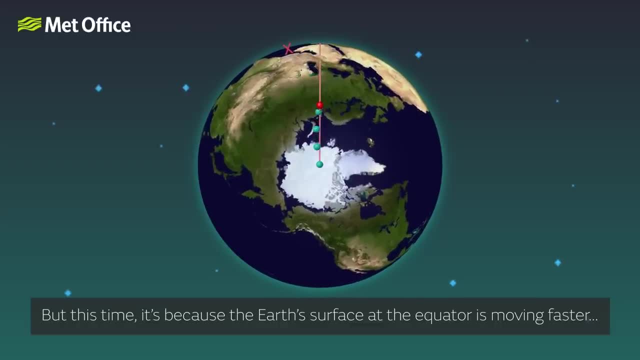 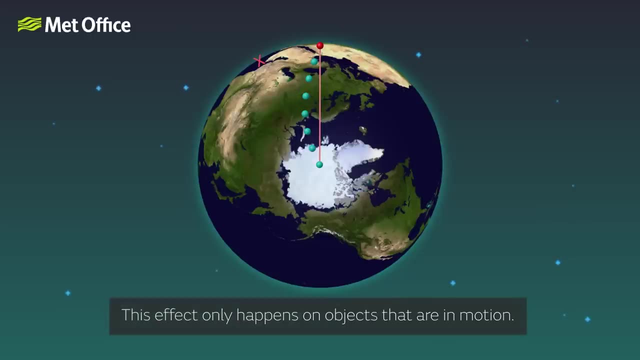 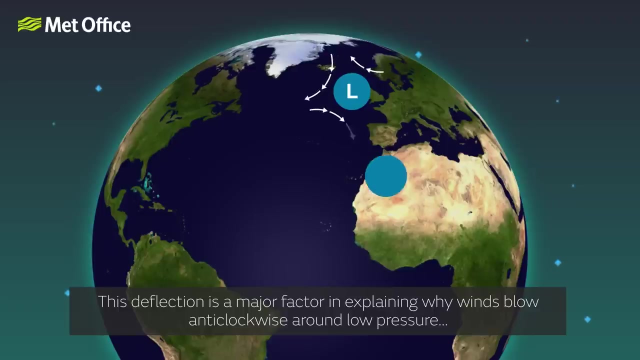 the Earth's surface at the equator is moving faster and has moved ahead of the ball. This effect only happens on objects that are in motion. This deflection is a major factor in explaining why winds blow anti-clockwise around low pressure and clockwise around high pressure in the Northern Hemisphere, and vice versa. 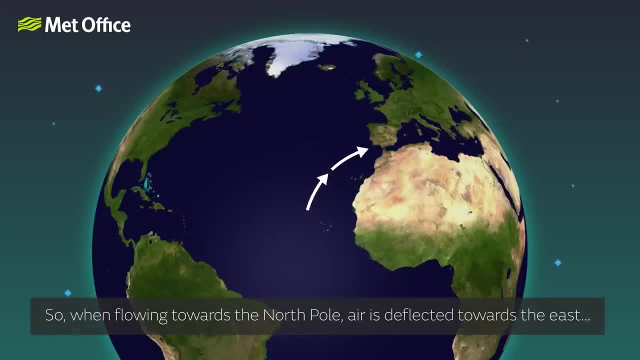 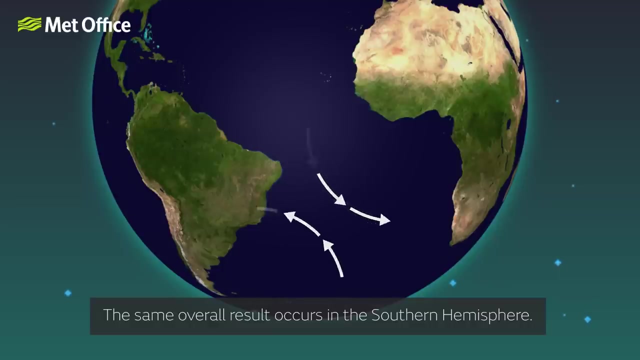 in the Southern Hemisphere. So when flowing towards the North Pole, air is deflected towards the east, and when traveling southwards, back towards the equator, it is deflected westwards. The same overall result occurs in the Southern Hemisphere. How does this lead to eastwards flowing jet streams? 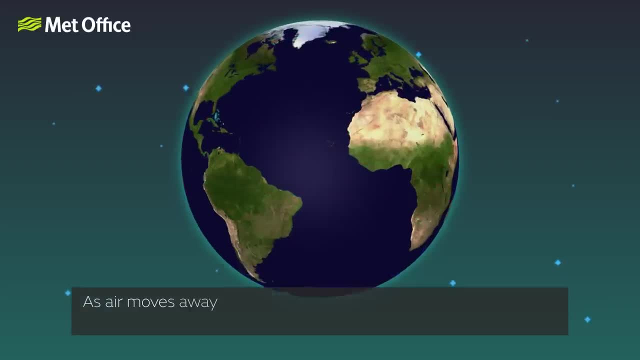 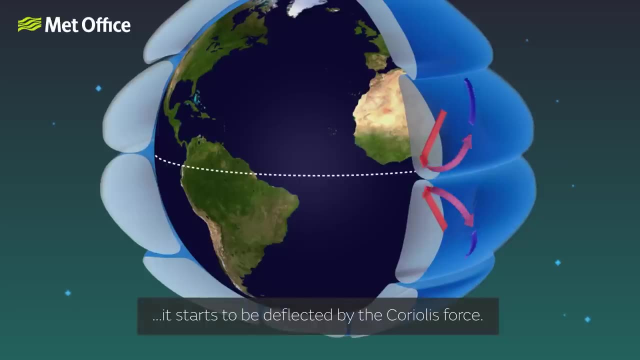 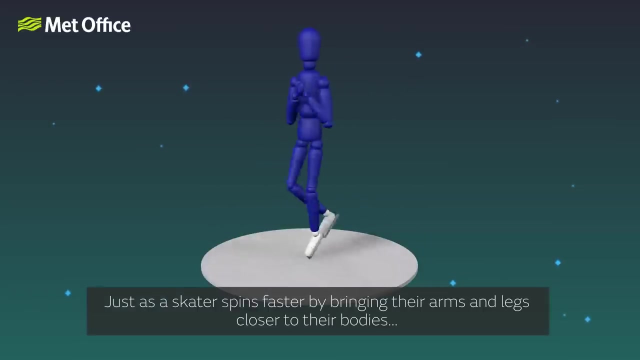 and prevailing winds. As air moves away from the equator, at the top of the Hadley cells, towards higher latitudes, it starts to be deflected by the Coriolis force. Just as a skater spins faster by bringing their arms and legs closer to their bodies, air moving away from the equator speeds up as it. 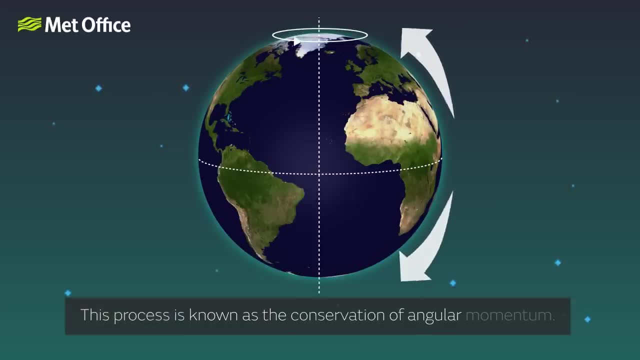 gets closer to the Earth spin axis. this process is known as the conservation of angular momentum- The magnitude of the Coriolis force increases towards the poles, so by the time the air reaches 30 to 40 degrees north or south, it is moving in an eastward direction. 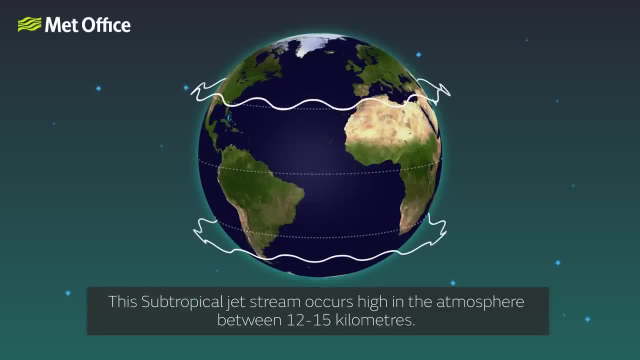 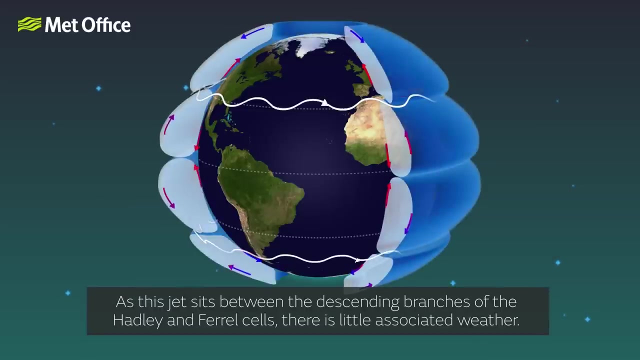 This subtropical jet stream occurs high in the atmosphere, between 12 to 15 kilometres. It is associated with some of the strongest winds on Earth, reaching over 280 miles per hour at times. As this jet sits between the descending branches of the Hadley and Ferrell cells, there is 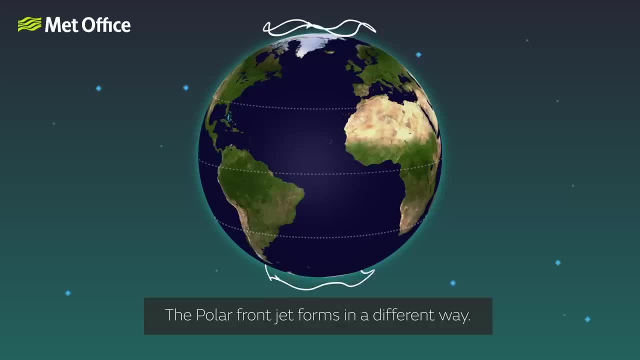 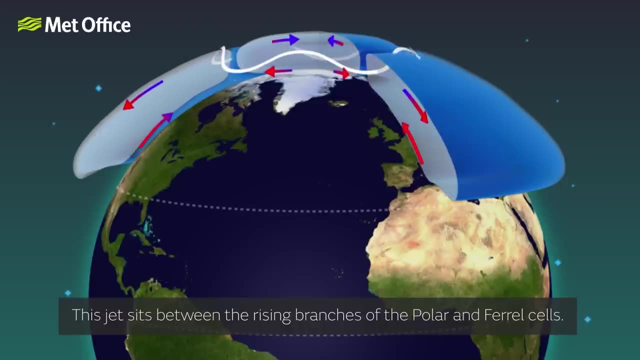 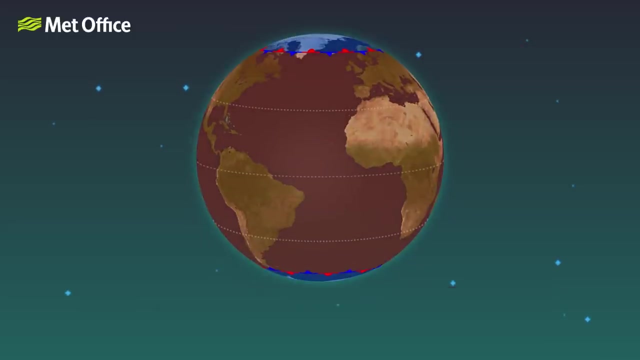 little associated weather. The polar front jet forms in a different way. This jet sits between the rising branches of the polar and ferrell cells. It marks the boundary between cold polar air and warm tropical air, known as the polar front. The polar front jet occurs at a height of 11 to 13 kilometres and is primarily used. 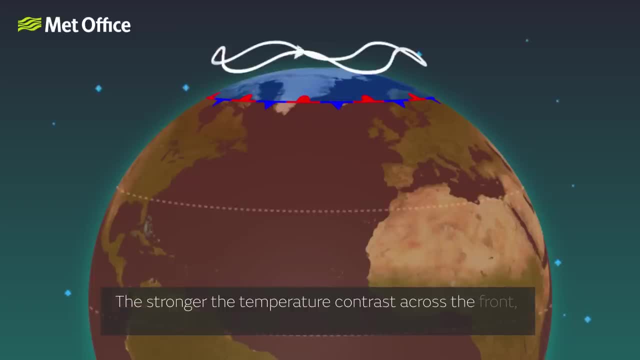 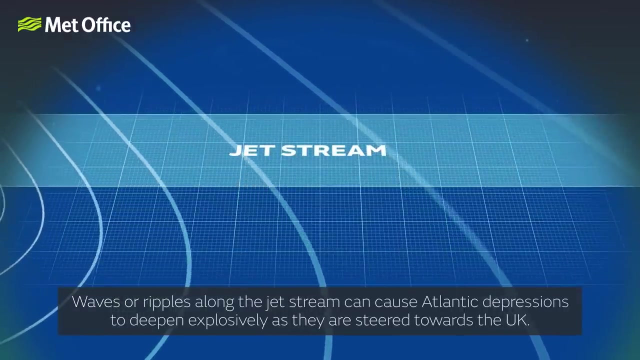 for temperature contrast across the polar front. The stronger the temperature contrast across the front, the stronger the jet. So it follows that the polar front jet is stronger in the winter than the summer. Waves or ripples along the jet stream can cause Atlantic depressions to deepen explosively. 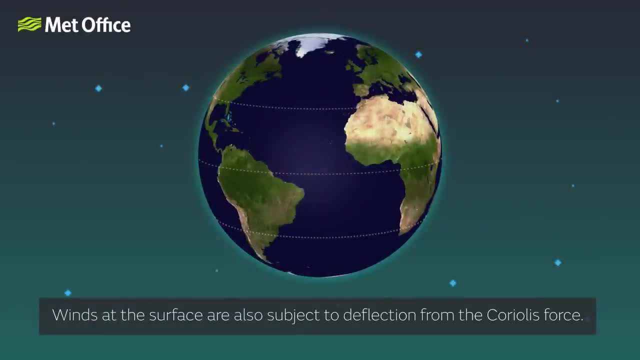 as they are steered towards the UK. Winds at the surface are also subject to deflection from the Coriolis force. The surface flow of the Hadley cells form the persistent Hadley force. This is the most common deflection in the Coriolis force. 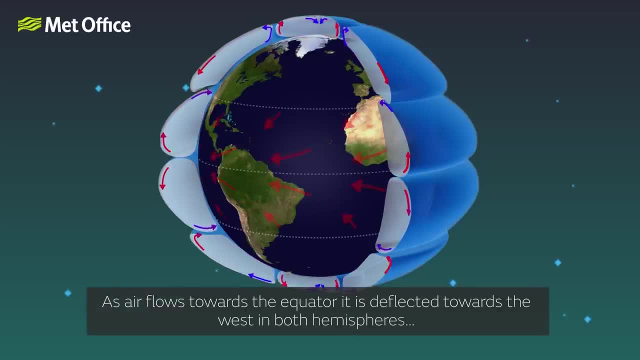 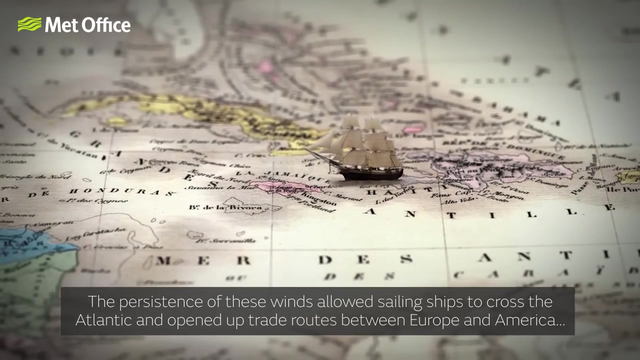 trade winds. As air flows towards the equator, it is deflected towards the west in both hemispheres, forming the northeast trade winds in the northern hemisphere and the southeast trade winds in the southern hemisphere. The persistence of these winds allowed sailing ships to cross the Atlantic and